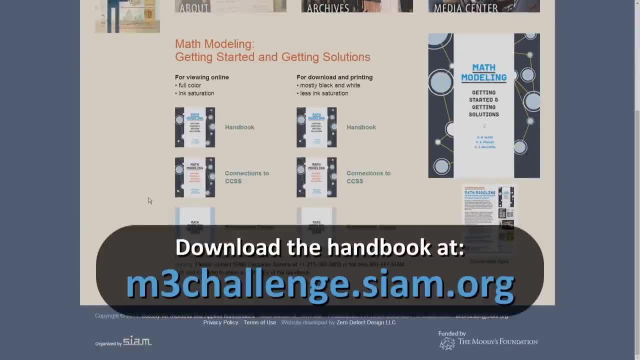 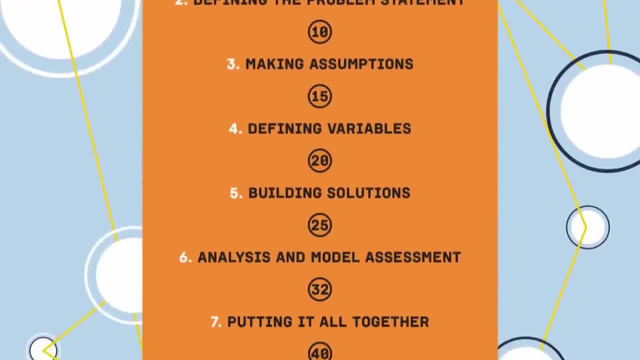 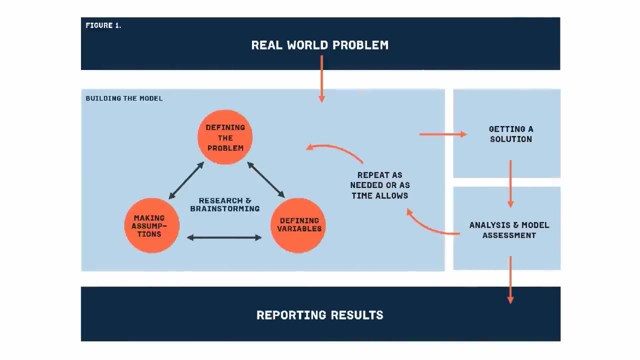 the Society for Industrial and Applied Mathematics created Math Modeling: Getting Started and Getting Solutions- a free handbook that provides a basic process for building mathematical models. We like to view the modeling process not as a sequence of specific steps, but there are different components that are revisited multiple times, and they include coming up with a concise 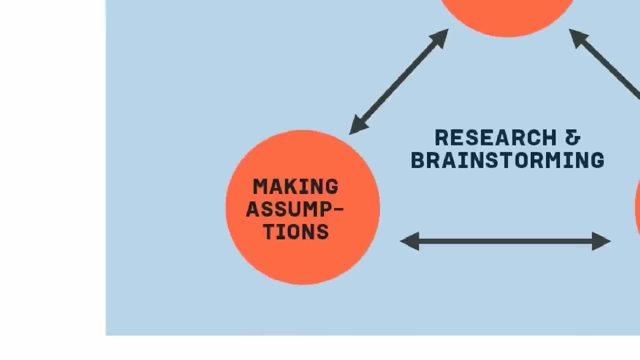 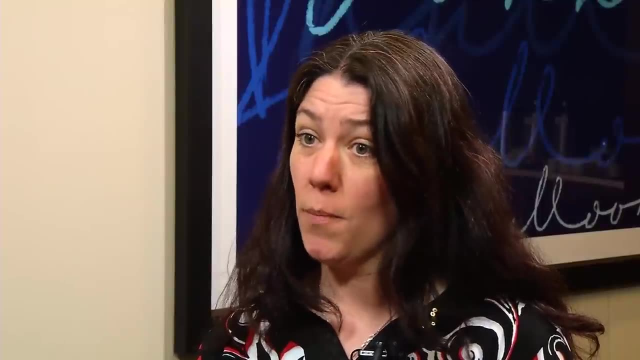 problem statement, making some assumptions about the problem that you're trying to understand, identifying the key variables in the problem So that you've got input and output to your model, what you want to measure at the end of the day- and then solving the model and analyzing your results. 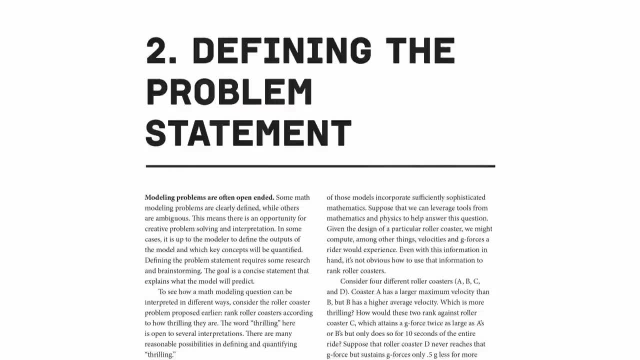 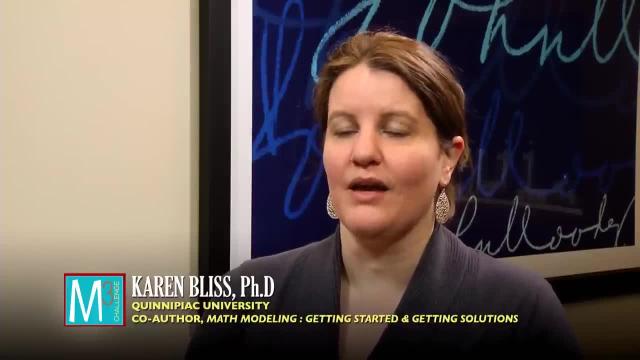 The first step in developing a model is defining the problem being solved. Figure out what question is being asked. So- and I know that that sounds simple, but a lot of times when you say, oh, I want the best way to do something, Well, tell me what. 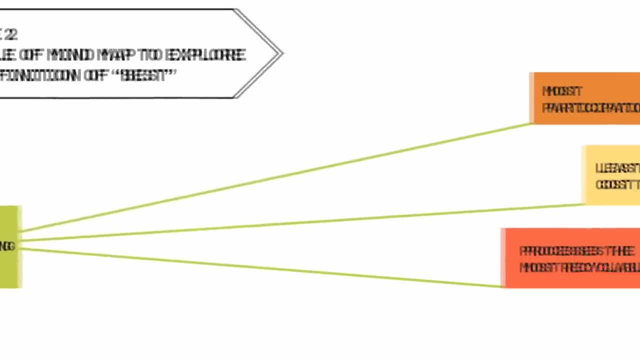 you mean by best? Do you mean the one that's the cheapest way to get it done? Do you mean the one that's the fastest way to get it done? What question are you really asking? Well, that's a good question. I think that's a good question. I think that's a good question. 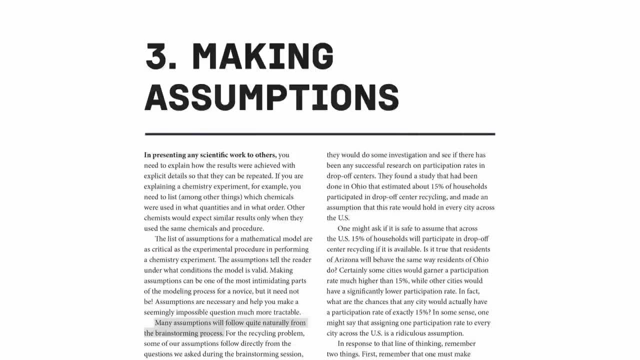 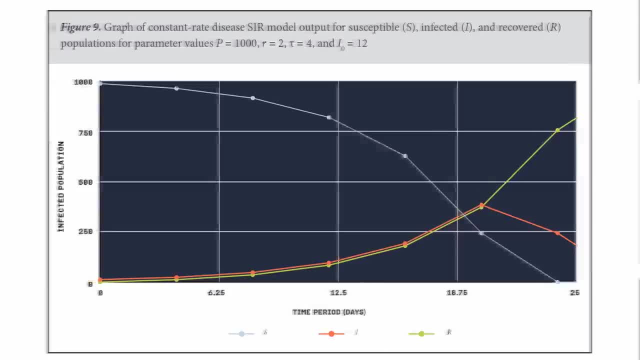 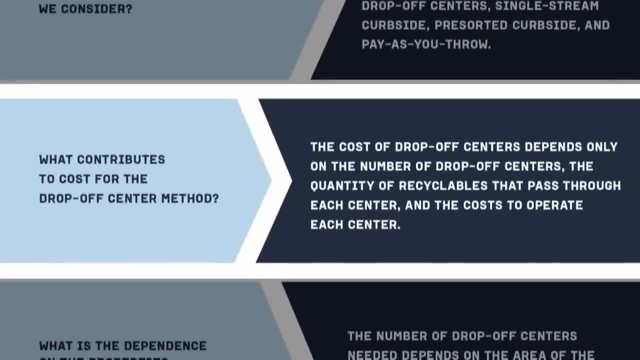 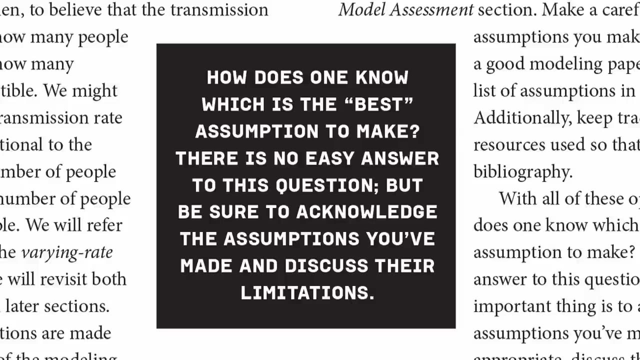 the disease spreads at a constant rate, versus some variable rate. When trying to find the ideal recycling method for a city, you might assume that only a certain percentage of people will participate in drop-off recycling. Sometimes these assumptions can be made based on prior studies or available data, and sometimes they are simply reasonable assumptions in the absolute. 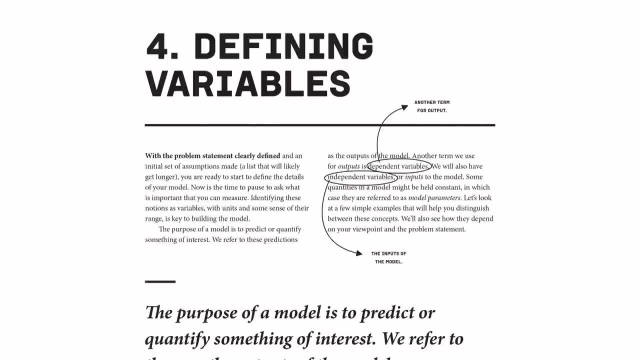 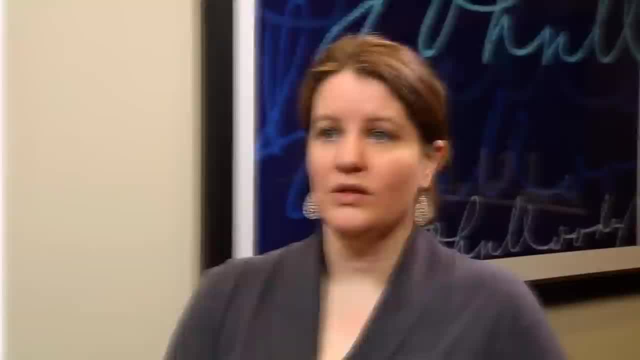 absence of data. Next is determining which inputs, quantifiable numbers and data can actually be measured, and how does the output of your model depend on those variables. Once I've decided what it is I'm trying to do, what sorts of things are my inputs and what sorts of things are my outputs? 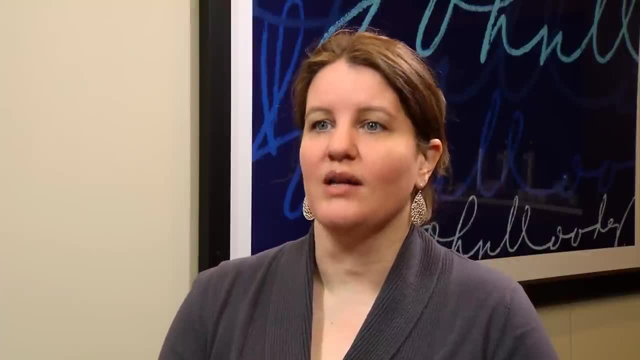 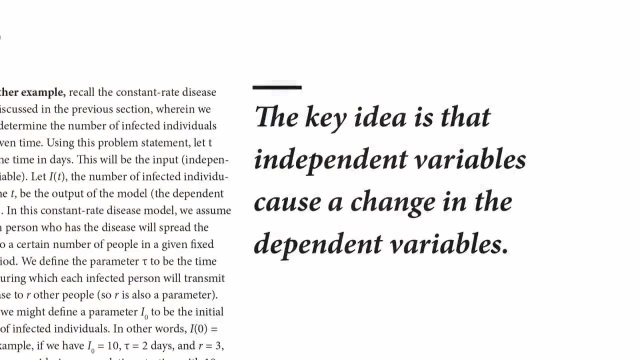 and I'm sort of the process of: okay, now that I know what I'm trying to get at, how do I quantify that? How do I get my hands on those quantities that I have control of those inputs, and how are they going to affect the outputs? 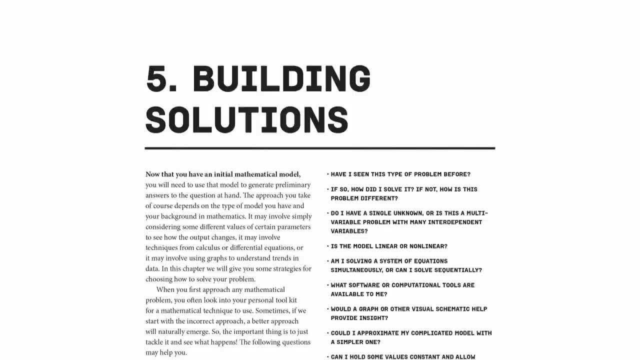 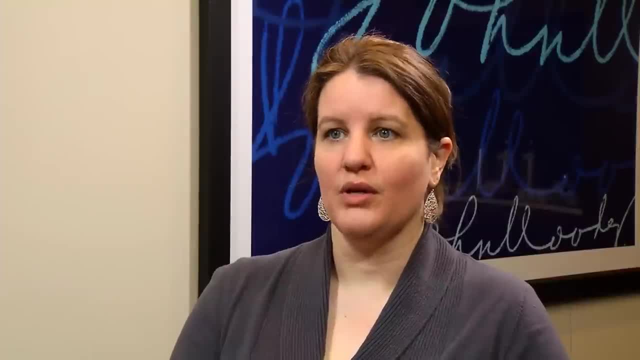 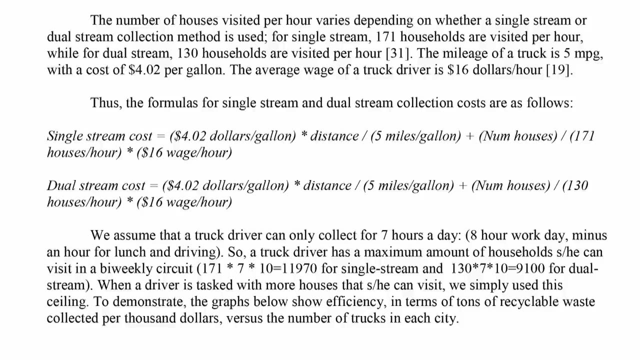 Once the question, assumptions and variables are in place, the next step is to build a solution using the mathematical skills and tools at your disposal. So you do some research and then you're putting together more assumptions and actually getting down to equations. I think this variable is related to this variable by this sort of equation. 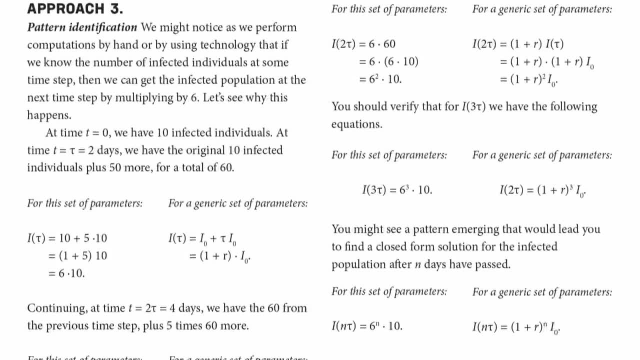 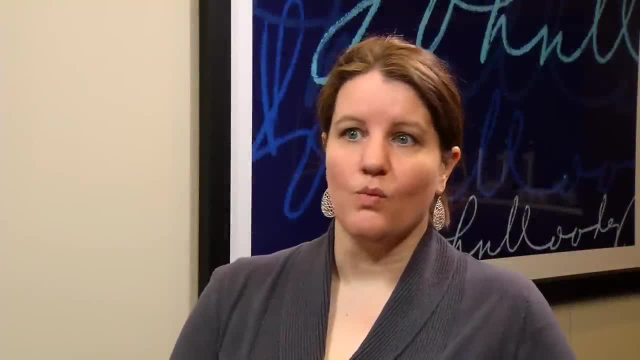 So, once you get your model together, you have now a set of equations, a set of inputs, a set of outputs. then you've got to figure out how to solve the equations, And again, this varies based on what your model is. 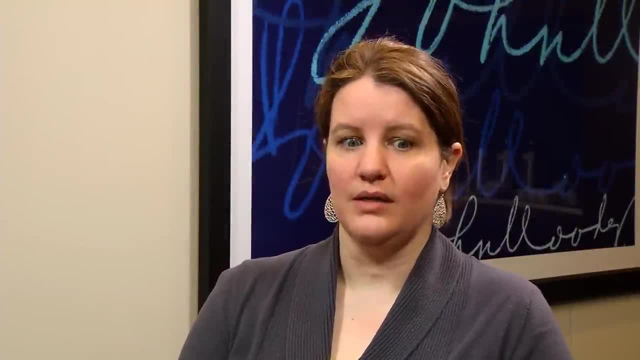 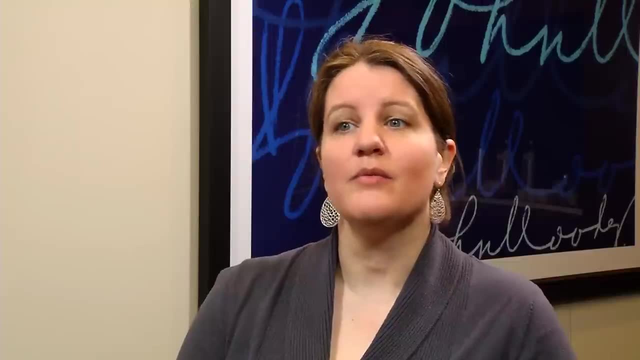 Okay, And what your skill set is. So if you're someone who you know does calculations by hand and with a calculator, that's great. So you'll do you know calculations by hand And maybe some of them you have to do some estimation. Totally fine If you're someone who has more. 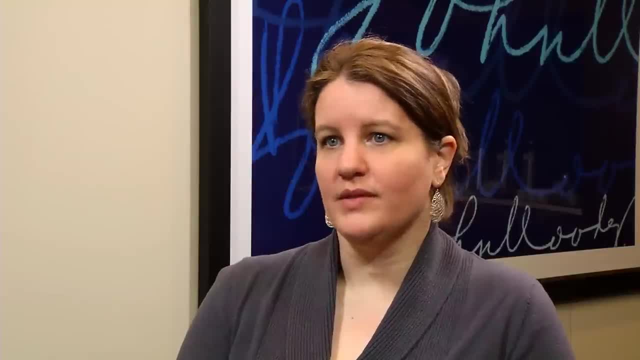 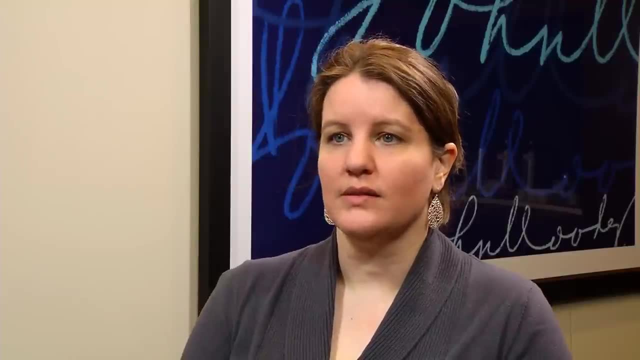 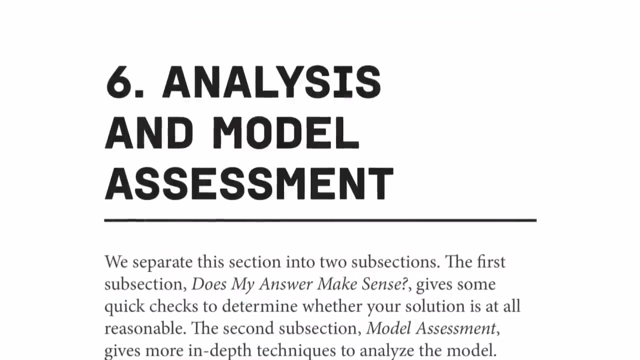 sophisticated tools, then you can perhaps take advantage of some software, So Excel, or you can use some of the open source programming languages. A lot of them are totally appropriate to solve differential equations or anything like that. A critical step in the modeling process is a systematic evaluation of the output that 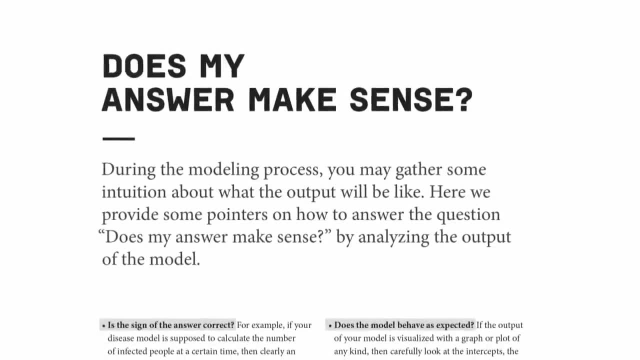 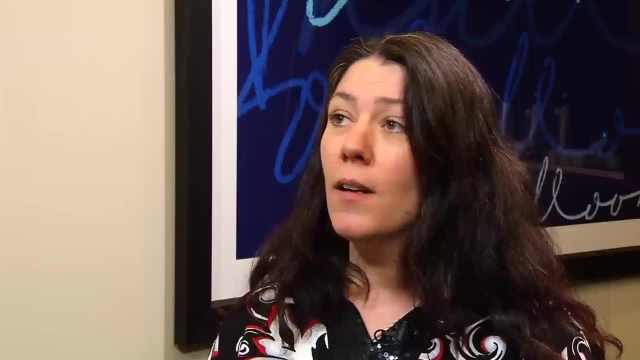 the model generates. One of the aspects that we really try to highlight in the handbook is that math modeling certainly does not lead you to one answer and one answer alone. There's a big difference between getting an answer and the answer at the end of the day. 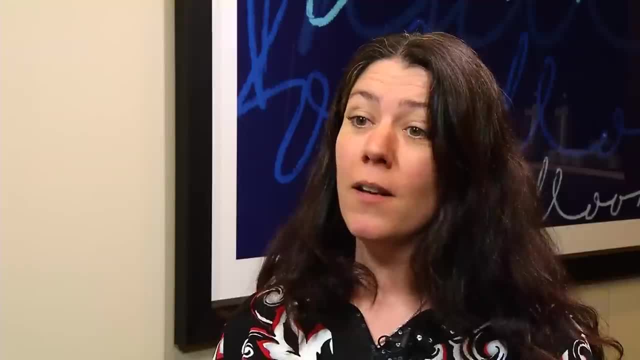 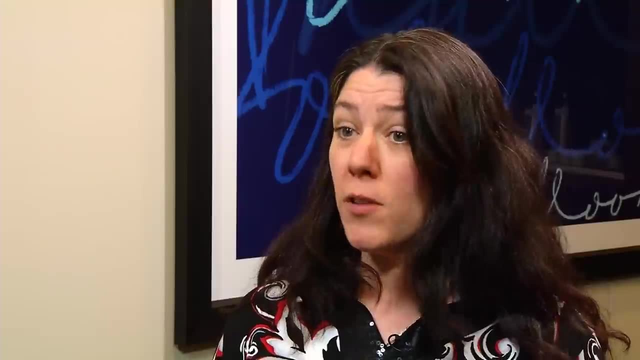 because when you're solving a math modeling question it's open-ended, So the answer at the end of the day that a student might get depends on the assumptions that they made at the beginning, So different groups of students would come at it from a different approach. 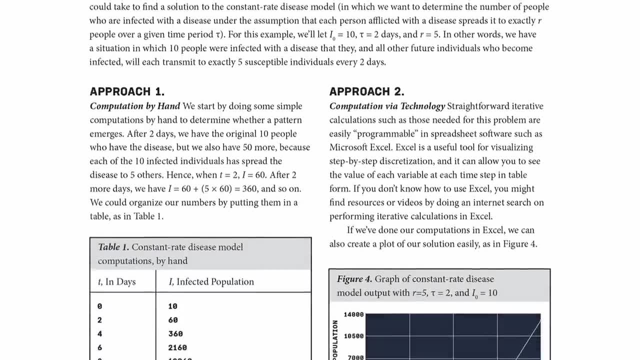 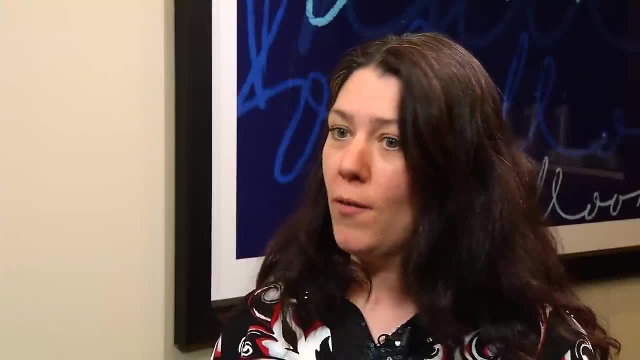 And a good example of that is a disease modeling problem. So if you were asked to predict how quickly does a disease spread, there's a lot of things that come into play with that, And one student may have a very simple model. You know, one person has it, gives it to two. 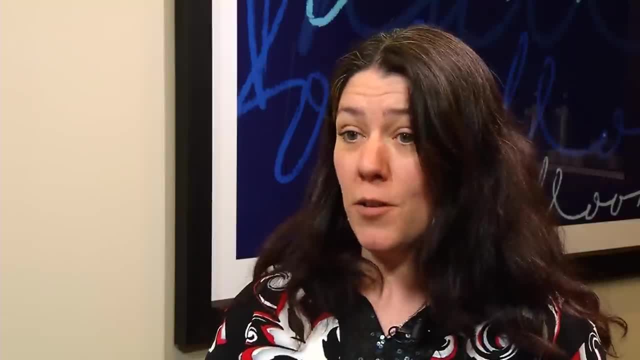 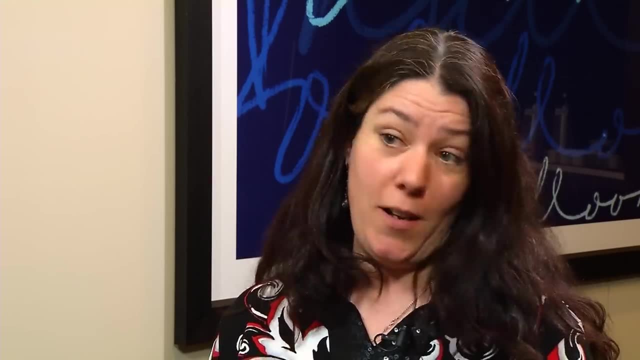 people every day. Those two people give it to two more people. That's an answer to that problem. that ignores a lot of realistic components to disease spreading, but it's still an answer. In defining the math modeling process we're really saying that. here's this thing that 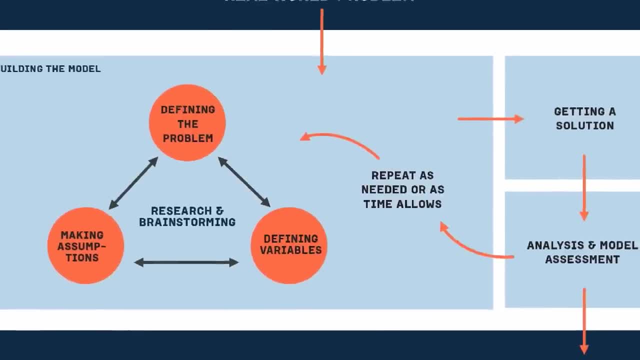 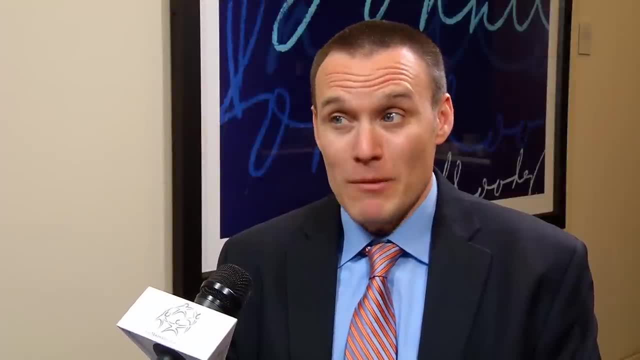 you're going to encounter. It's not a set of steps in which you're saying: oh, I've done step one, I've gone to step six and now I'm done with my model forever. In many cases, when you're dealing with real-world problem solving, you are expecting to encounter a 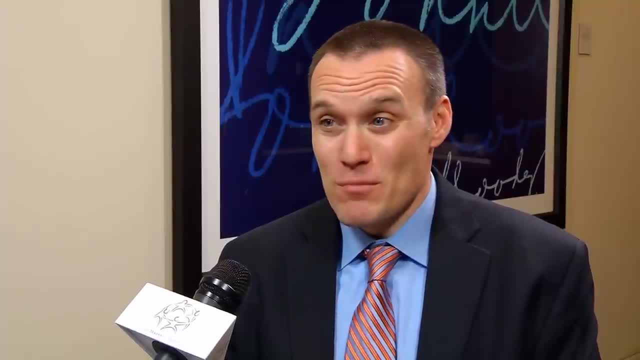 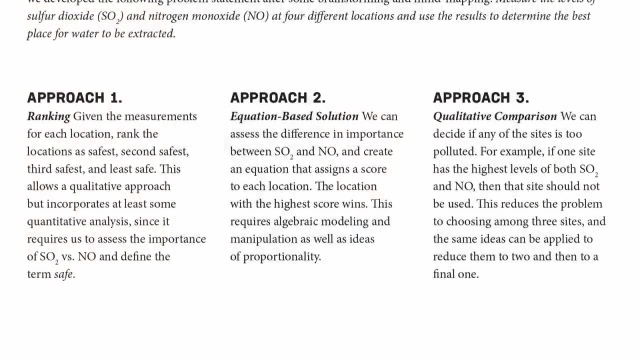 variety of solutions And, in fact, I would argue that if you only have one solution, your answer is less believable. And one thing I emphasize throughout math modeling, saying that you want to find an answer. Well, once you find the answer, you're going to have to find a solution, And that's what 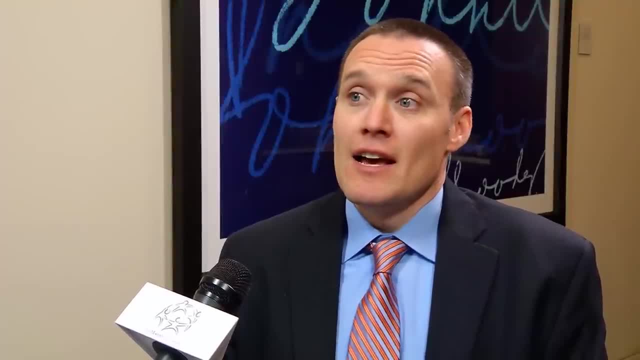 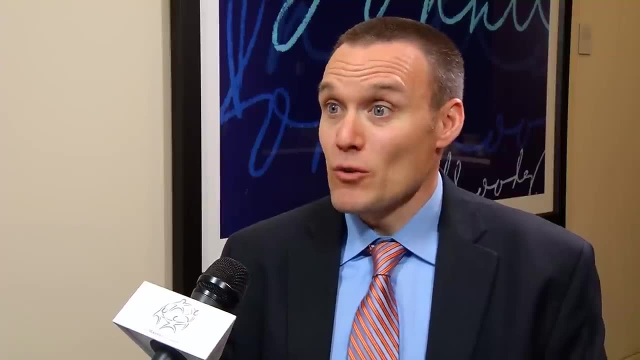 it's all about. You want to find the answer, You want to analyze the answer, You want to communicate the answer And then, probably through that analysis process and talking about it with others, you're going to realize: wait, there's other ways to do this, Or there? 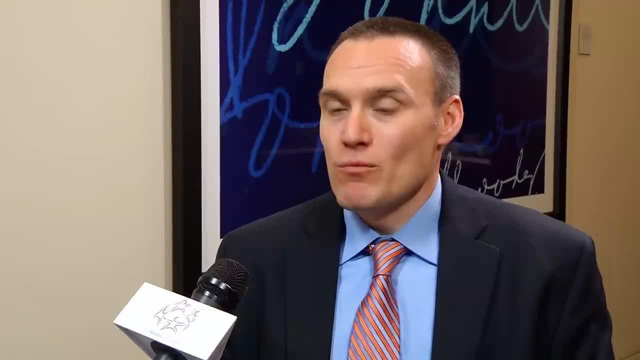 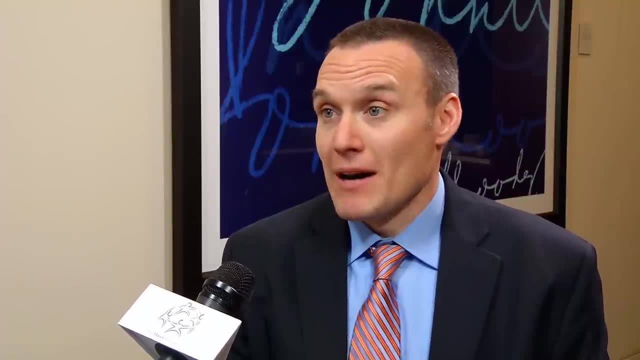 are ways that there are things we made assumptions about that. we realized we could change those things and now we have a stronger model If we went back to this other part of our model, made a switch here, made a switch there, and now we have a different solution, or maybe. 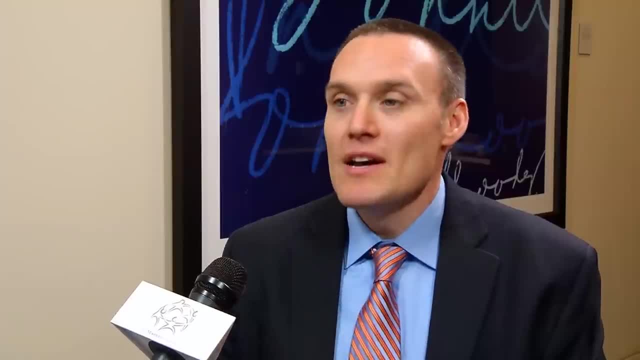 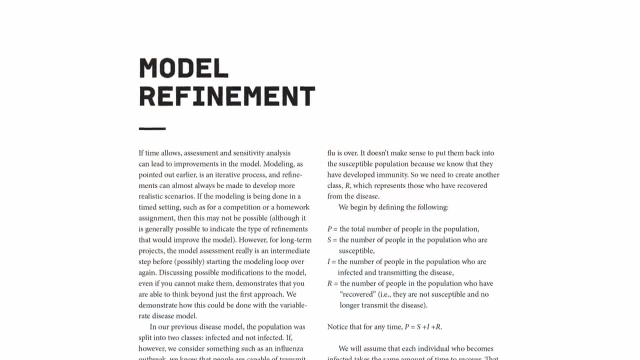 we find out that it's the same solution, So we have a really strong solution. So you're going to continue to move throughout this process. I would say you cycle through it, And that would probably be a way that I would describe the process, as opposed to the steps that are incorporated into modeling. 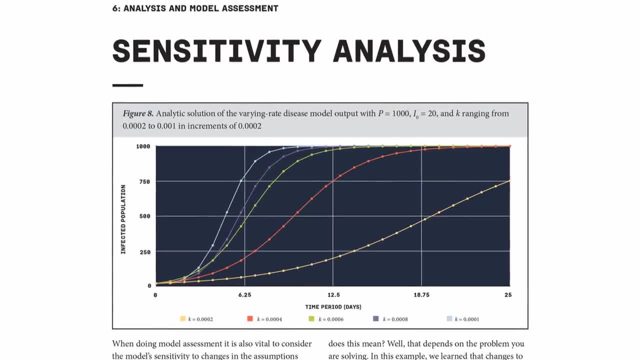 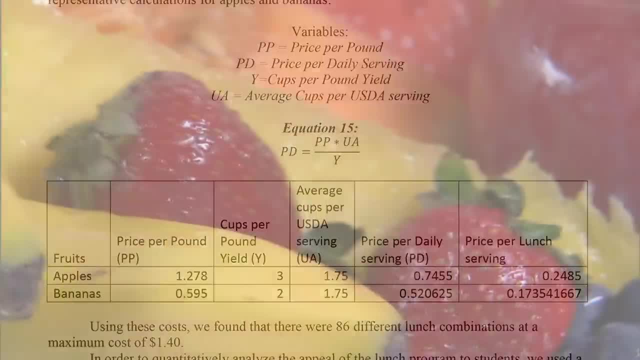 Another vital step in model assessment is to analyze how changes in the assumptions and parameters affect the model's output. For example, in a model used to predict the cost of a school lunch, does a minor change in one input say the cost of fruit have? 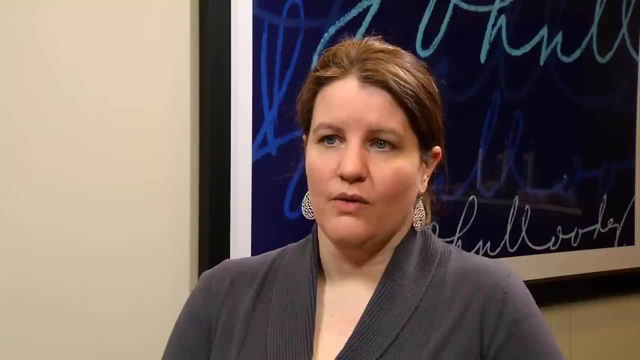 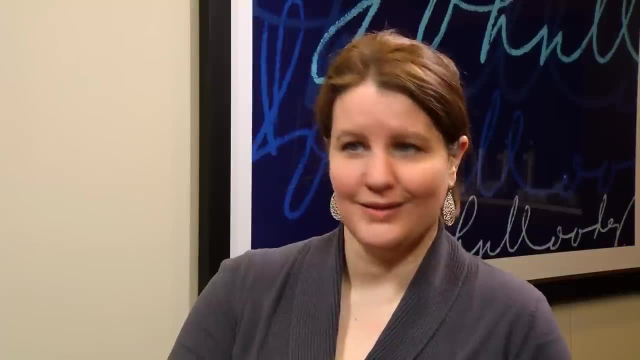 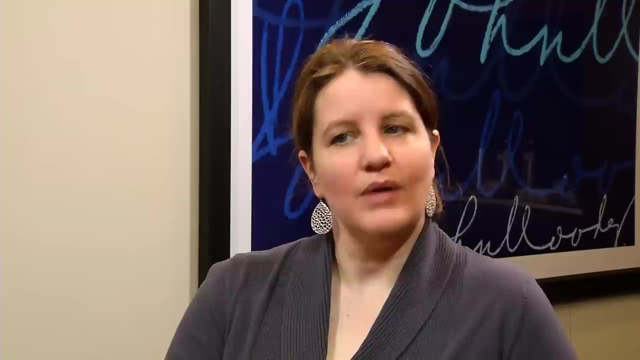 a small or large impact on the model's output. So I know that we need to have this much fruit and this much vegetable and this much whatever, And I've assumed that fruits cost this much And we have to make assumptions in order to get an output for our model, but I don't really know that that's how much fruits. 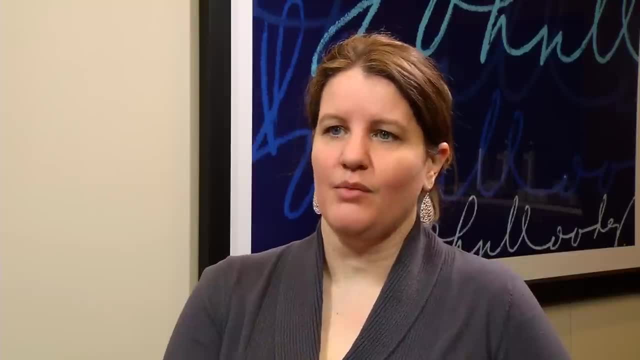 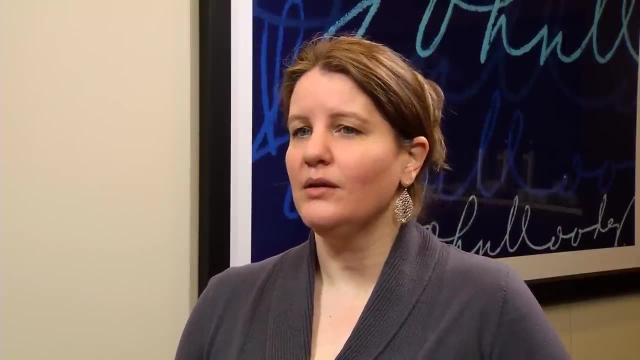 cost all the time year round. So if I play with that number a little bit, if I make it a little bit bigger, a little bit smaller, does that make the change in the total cost of lunch a little bit bigger, a little bit smaller? 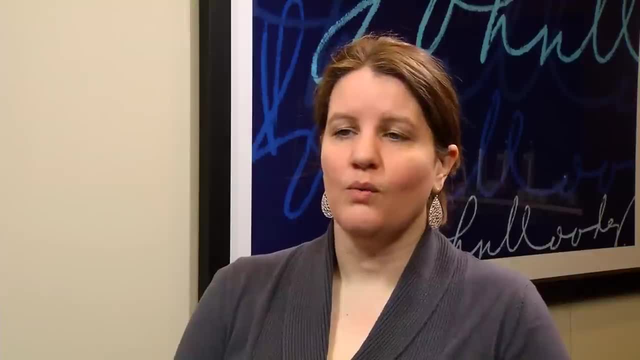 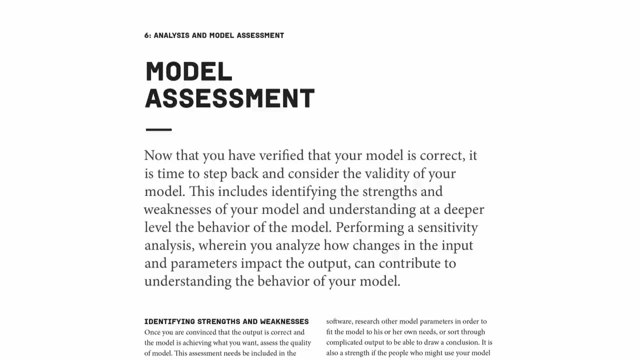 Yeah, it does. It does make the change in the total cost, make the answer totally wildly different. There's an important step at the end of the modeling process that comes with analyzing your results, And there's a great deal of honesty in that in terms of linking your solution.